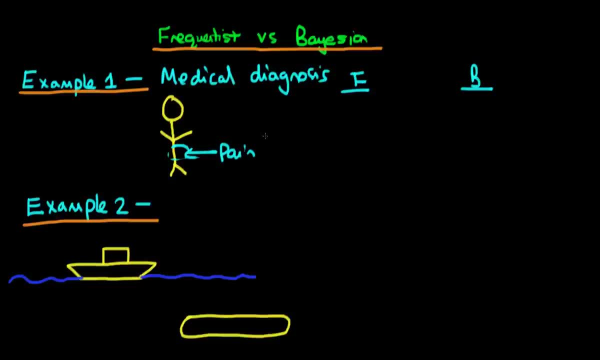 first think about the frequentist approach to diagnosis. How would that work? Well, the idea is that the doctor would have some sort of model for the cause of this particular pain, and this is some sort of mental model which could explain all possible causes of a stomach pain. And then what the doctor 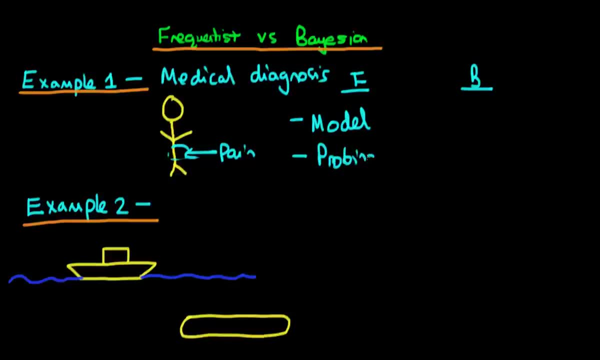 would do is perhaps by feeling your stomach, perhaps by probing with his fingers and sort of getting your feedback. he would then use that sort of sort of feedback as an input into the model, and that would then help identify the source of the pain. So the idea here is that what we're purely doing is we're 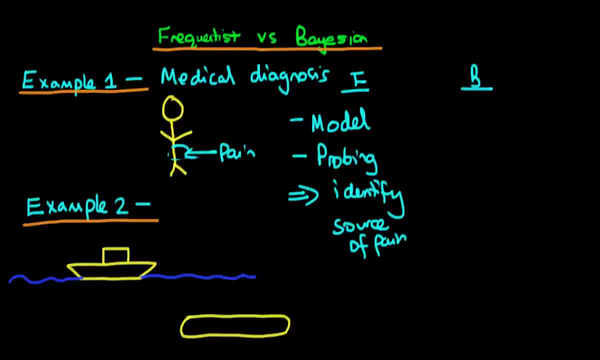 using the sort of information which is available to us at the time by doing this sort of probing. Okay, so how would this differ with the Bayesian situation? Again, a Bayesian statistician would have a model for sort of identifying the causes of stomach pain, but the Bayesian doctor 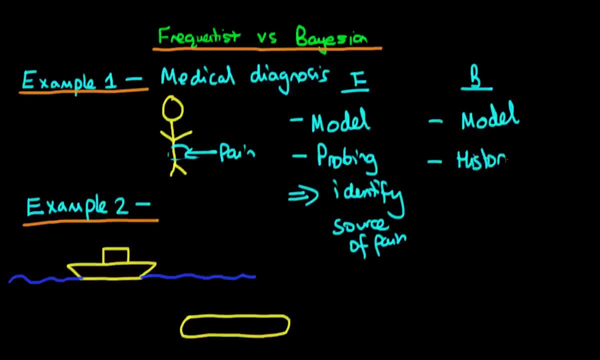 would also have to hand a history of the patient, So that history of the patient might be. you know, it might include, for example, this patient has had pain in their stomach in the past. Then what they would do is they would then sort of probe and again get feedback and then he would use this as an input to the 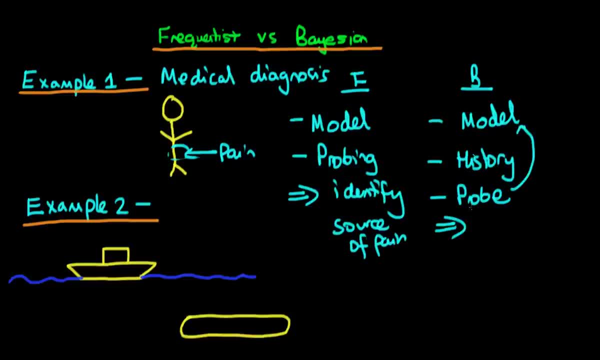 model, and he would also combine that with the prior history of the patient. So it's this combination of the sort of model results, together with the prior knowledge of the situation, that then helps them to identify the source of the pain. Okay, so that's the example of medical diagnosis. The second example: 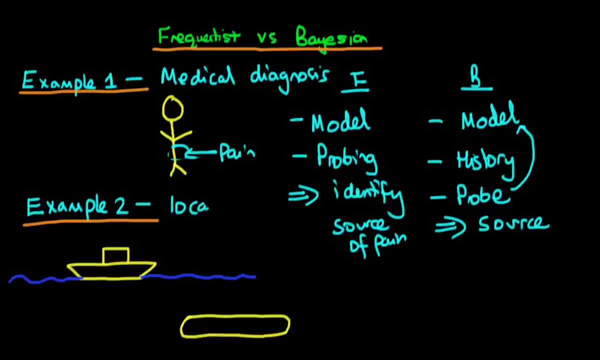 which I want to talk about is if we're trying to locate a submarine, So we assume that we're in the middle of a submarine and we're trying to locate a submarine, So we're in this ship up here and what we're doing here is we're. 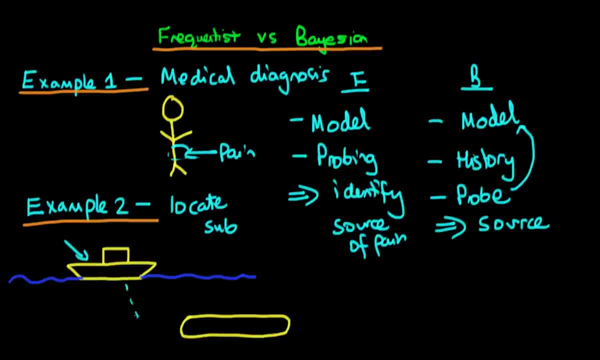 using echolocation. So we are sending out sound waves from the bottom of the ship and then we're sort of waiting to hear how long it takes for that particular sound wave to return back to the ship. So we've got all these measurements on, let's say, the length of time it takes these particular sound waves to return. 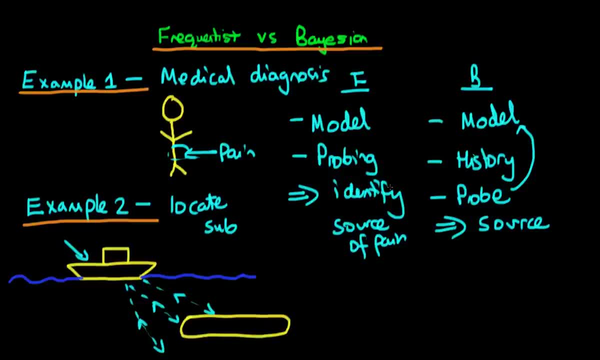 and we're going to compare how a frequentist would view the situation and use that to identify the location of the submarine and compare that with the approach. So again, if you're a frequentist, what you would have is you would have a model and this model would be a sort of